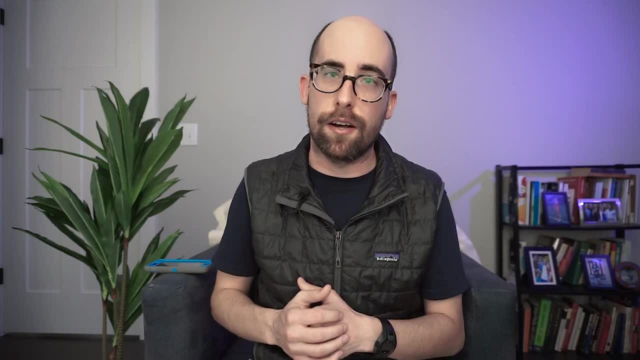 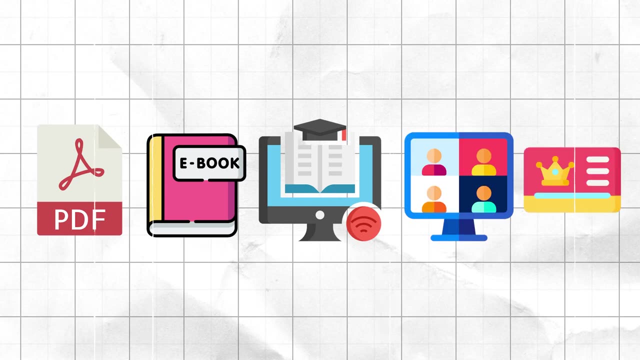 you make it once and you can sell it infinitely, and I think that's pretty awesome. Examples of things you could sell here are pdfs, ebooks, courses, cohort-based courses, courses, memberships- the possibilities are really endless. but, as I mentioned, it's a 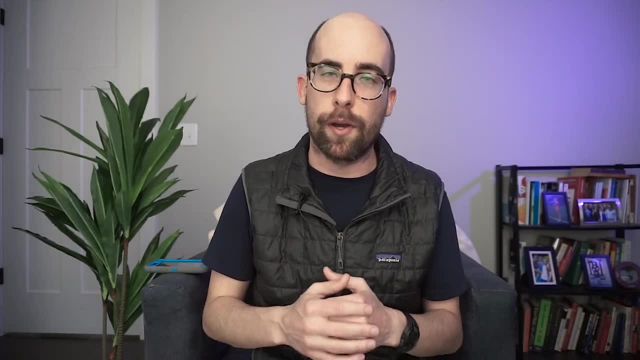 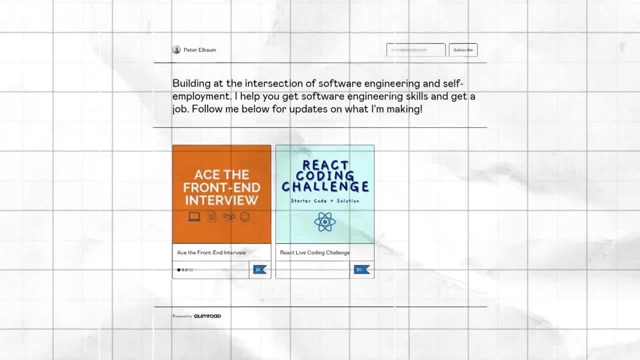 lot easier to make significant money selling info products when you already have an audience And full disclosure for me. I have two products on Gumroad right now- One is free and one is paid, and they're both kind of eBooks but they have video components. 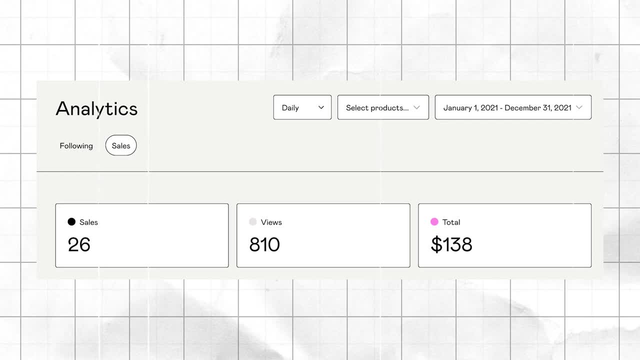 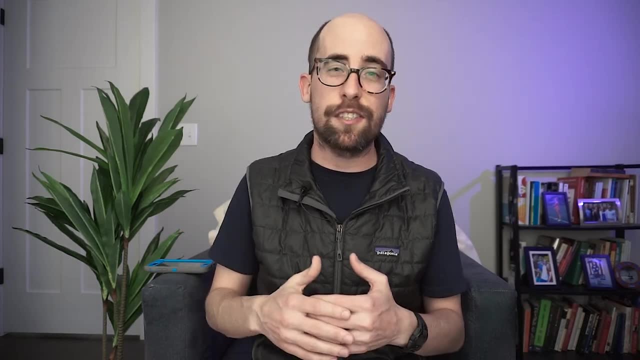 with them And last year I made 26 sales for a total of $138.. So, as I mentioned, it's hard to achieve enormous scale unless you have a significant audience, because these are kind of one-off, not recurring purchases, but it's totally passive, like 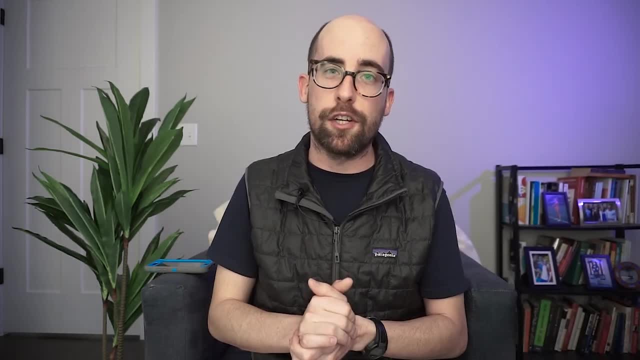 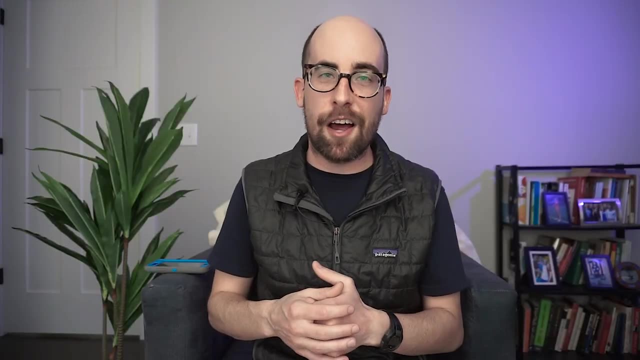 I mentioned, And I think it's a pretty great revenue stream if you can manage to get it in front of people and have a decent conversion rate. Okay, Our second idea, and that is blogging. Now, blogging may sound a little old fashioned and you may think that the day of the blog 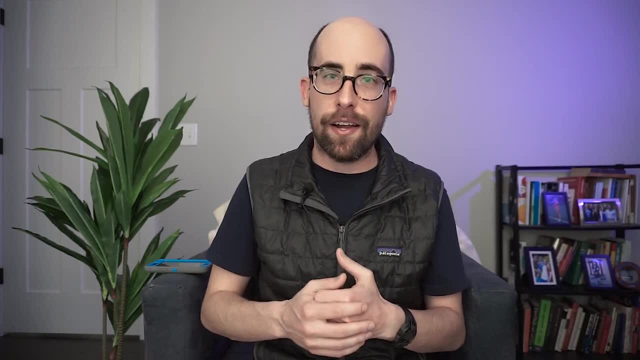 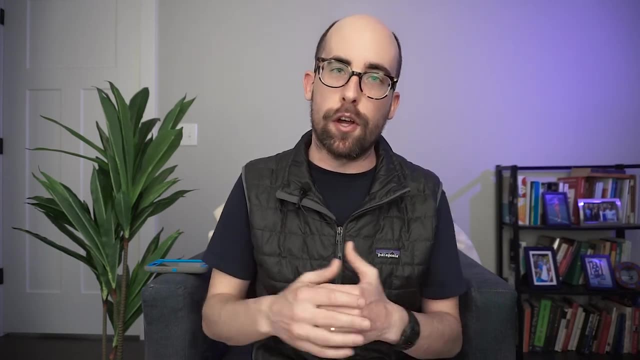 is kind of gone, that we moved on to other things, but I think having a solid blog with really valuable content, with backlinks and SEO traction, is incredibly valuable and shouldn't be overlooked. A blog is valuable for a lot of reasons. I think number one: it can help you establish a personal brand. 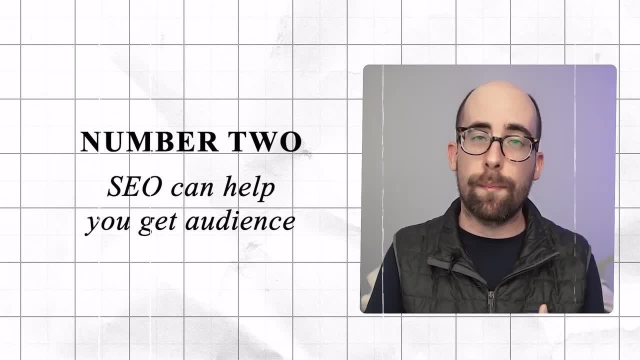 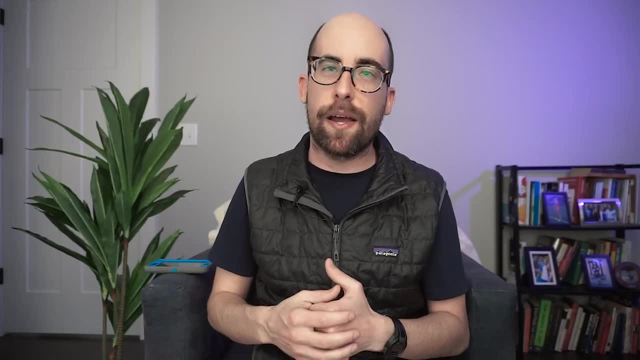 And number two, if you can get some of that SEO traction I mentioned, then that could be another source of kind of getting your thing in front of people. So I'm not a blogging expert, but I do have a few ideas in this space. 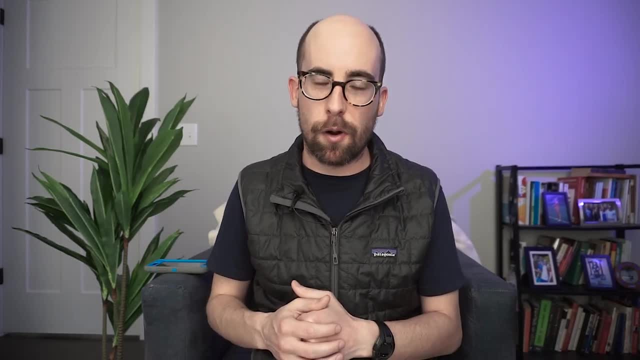 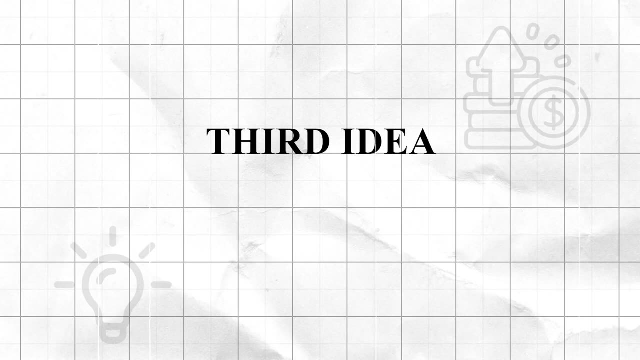 And so maybe I'll circle back around and update you guys once I launched these projects, But suffice to say for now. don't overlook blogging when you're thinking about ways to make passive income online. Our third idea is related to blogging, and that is affiliate sites. 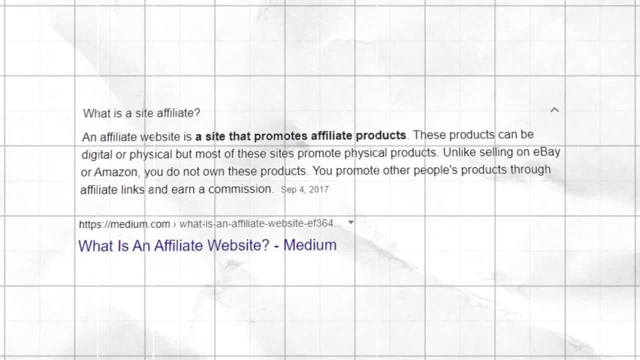 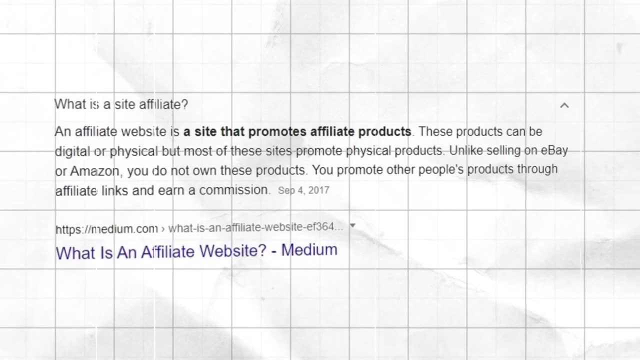 And what are affiliate sites? So affiliate sites would be sites that are centered around a certain class or type of product, that maybe review that product and then have affiliate links in the blog posts that people click through. Now the thing with affiliate sites is you need significant traffic in order to make. 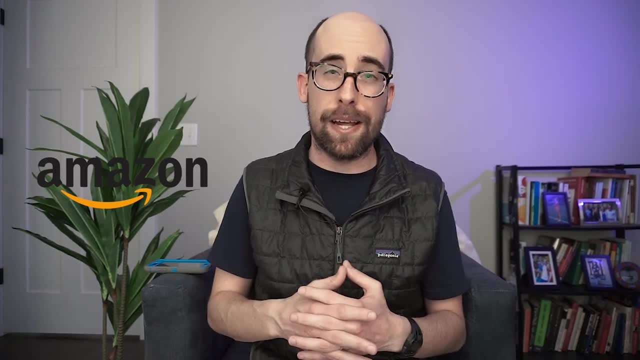 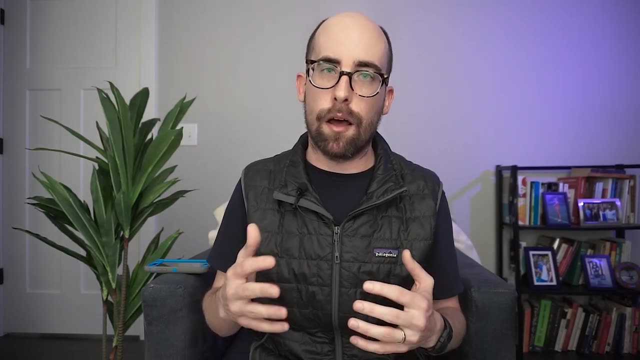 any kind of decent money, because Amazon's affiliate program pays pennies on the dollar. I don't think it's very significant from what I've heard, but I think these are still pretty good ways to make money online, And so I think, as an example, the foremost 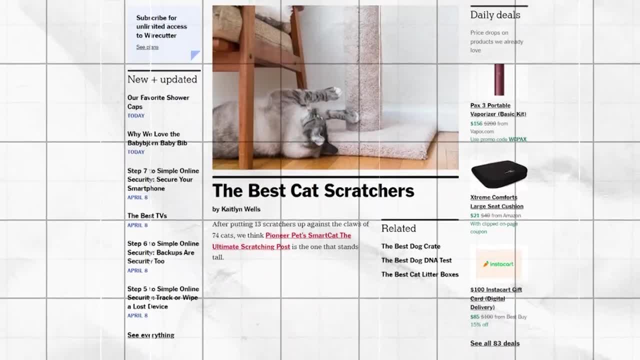 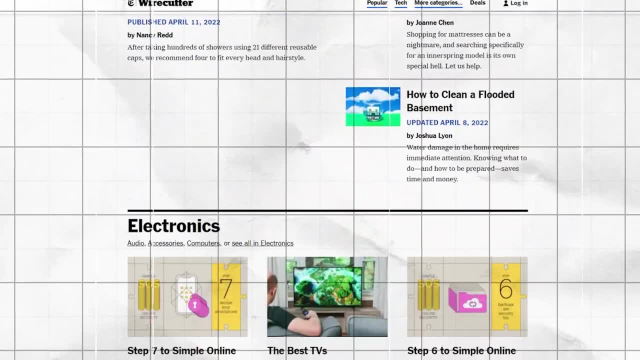 Kind of example that most people would know is Wirecutter, which was bought by the New York times, And so Wirecutter did reviews of products and kind of bought everything, kind of relentlessly tested these products and had basically the gold standard for product reviews and they 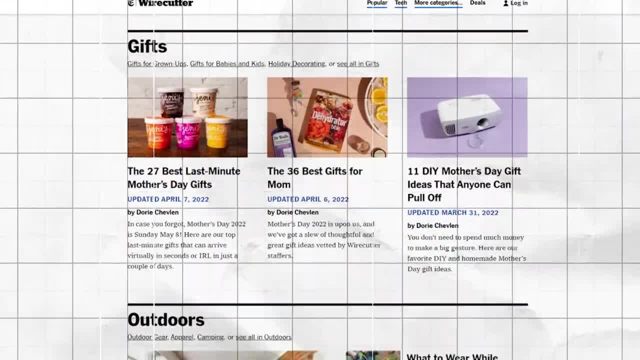 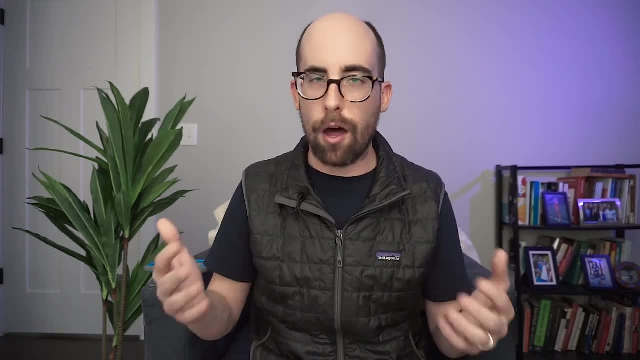 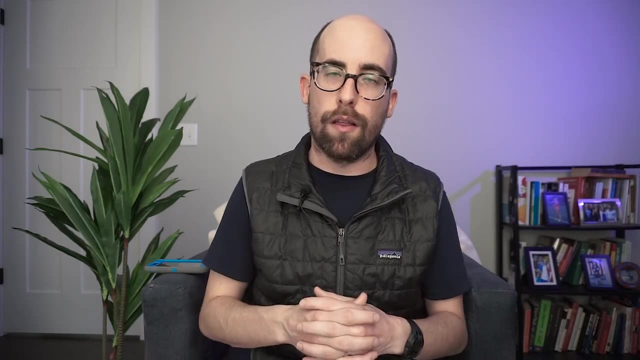 monetized in part through affiliate links, And so that's just an example. but you can niche down infinitely on these, So you could do a blog reviewing boats or reviewing lawnmowers or grills or really anything, And If you're looking for a niche affiliate marketing website would be a pretty good way for a lot. 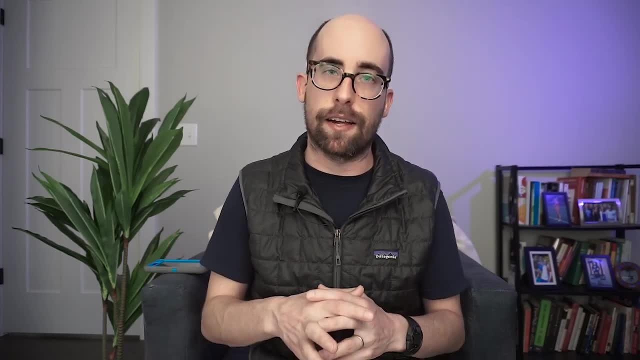 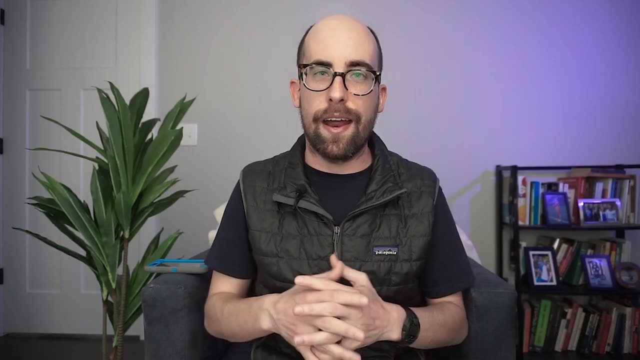 of people to get started, And you can also acquire these on websites like Flippa. So consider that when you're thinking about passive income strategies. Our fourth passive income strategy is YouTube, and YouTube, I think, is not a secret to most people at this point. 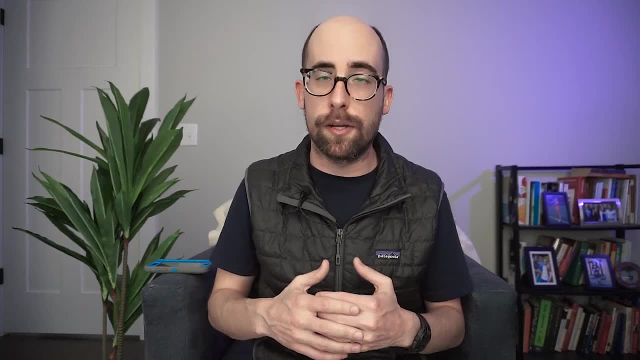 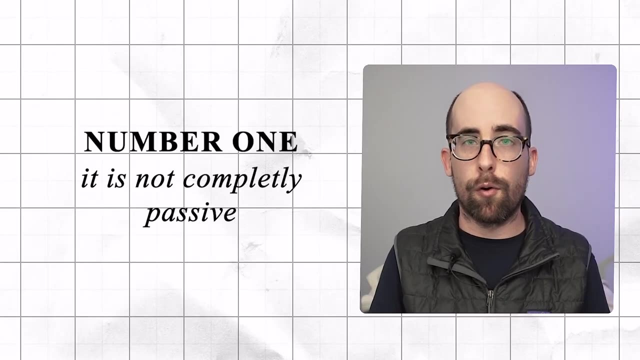 You monetize it through a lot of the means that we've already mentioned, So principally through ads and through affiliates. And the thing about YouTube is number one: it's not completely passive, because in order to kind of keep your channel healthy And continue to drive views, you need to be continuing to make videos, like I'm doing. 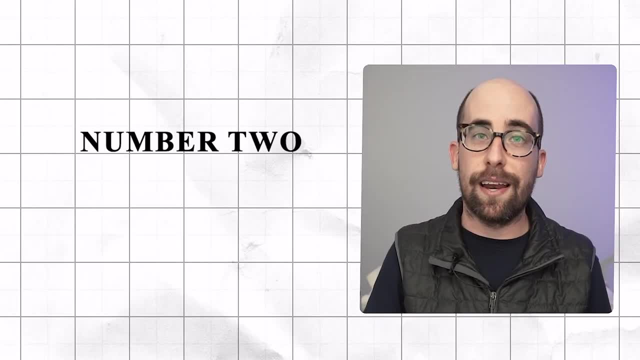 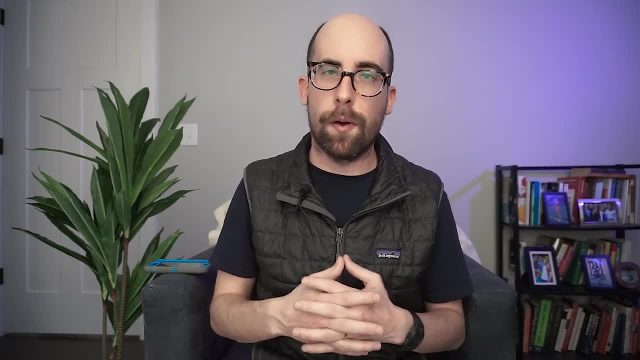 right now, And so that's part of it, And the other part of YouTube is that it's an extremely long game. So no, for me personally and for most people, it takes tens, maybe not hundreds, but maybe over a hundred videos to see any kind of significant traction. 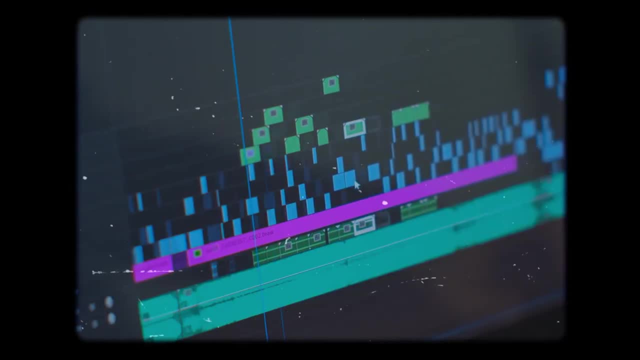 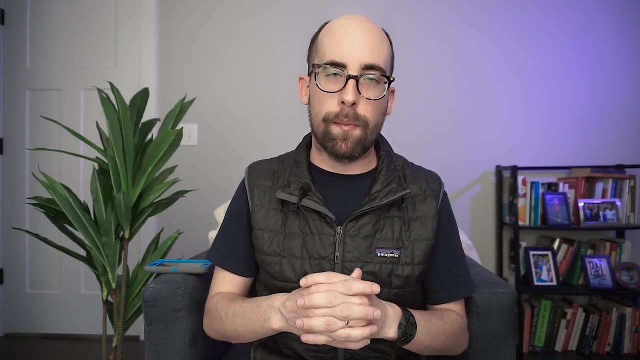 Most people, when they start out, don't know anything about cameras. I didn't don't know anything about editing. I still don't know that much about editing, And so it's tough. in a nutshell, it's tough And so. 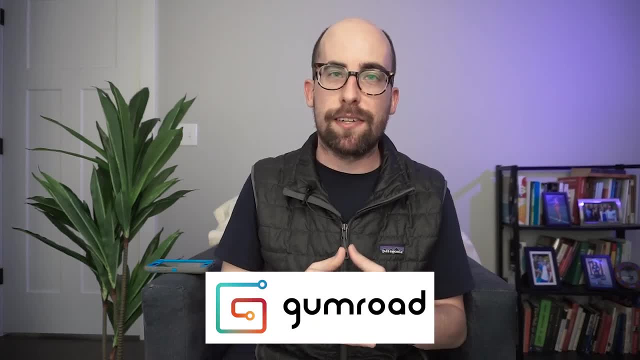 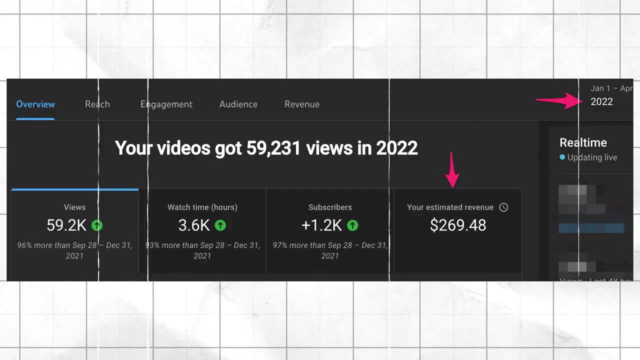 I'm not realistic about that for people and kind of like gumroad: unless you have a significant audience, it's hard to make money at YouTube. So just looking at my analytics here, I was able to monetize in late January of 2022.. 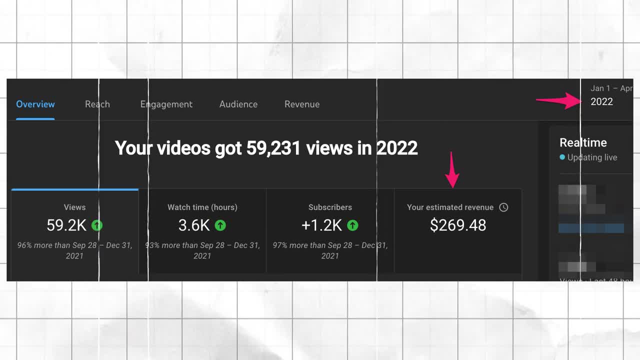 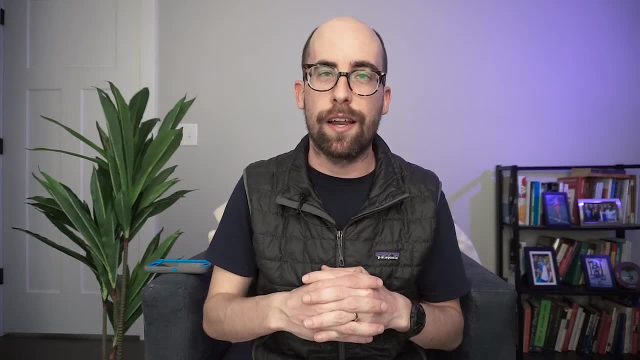 And so far, I'm filming on April 6th and I've made $269 and 48 cents. So you can see it's tough to make significant money on YouTube, like I mentioned, And so it's an interesting revenue stream. I think it's brought a lot of interesting things into my life, and allow me to meet. 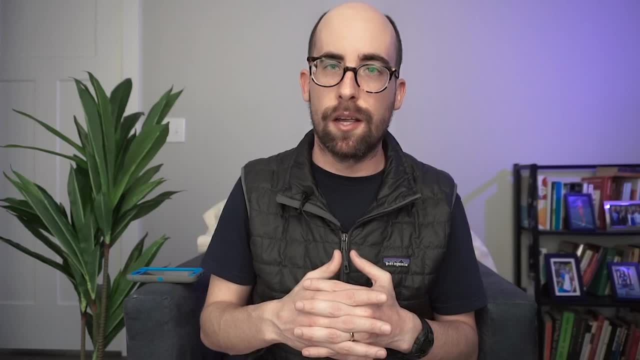 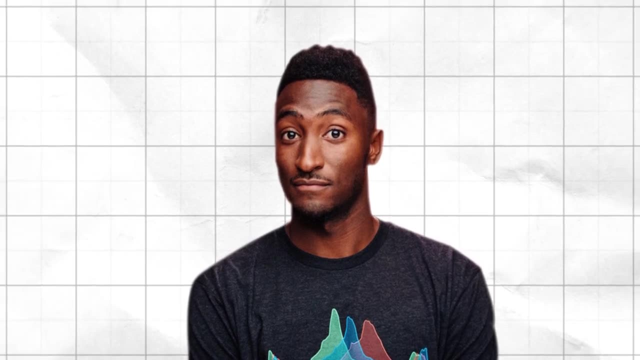 Interesting people, But as a significant income source. you're not going to be making a full-time living on it, Unless you're like MKBHD, whose channel is mostly funded by AdSense. When you are in kind of those tech and personal finance spaces, the amount that YouTube pays 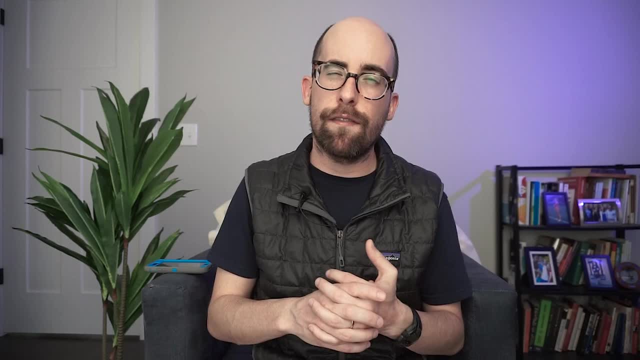 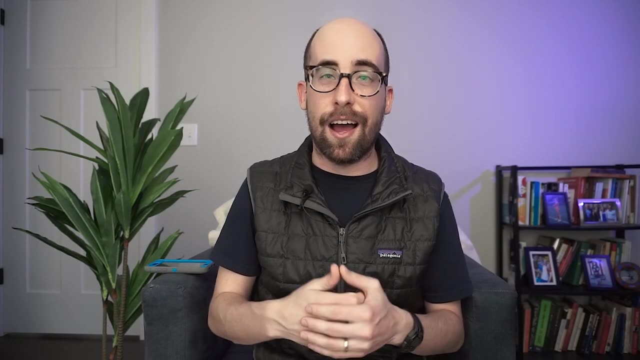 you for ads on your channel is more typically, And so it kind of depends a little bit on what niche you're in. but the long story short is that this is just tough. It's tough to compete, and I do it because I really enjoy it. but I just want to be realistic. 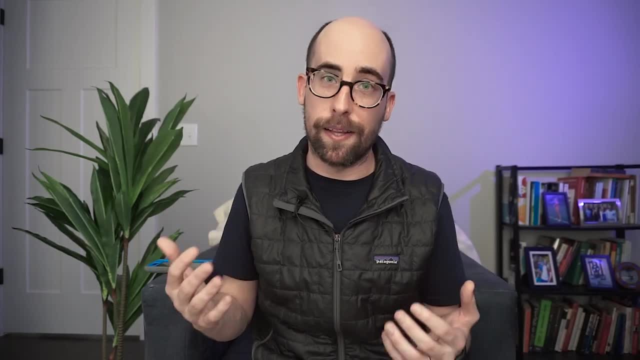 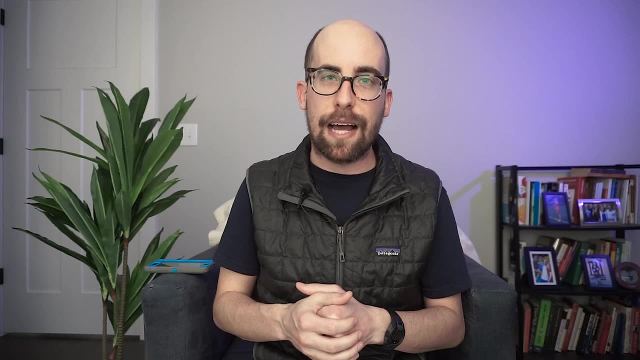 About what the struggles are like and the fact that it's not completely passive. Our fifth passive income idea is the Holy grail for developers, And that is building a SAS. talked about building a SAS in the past and it's the Holy grail. 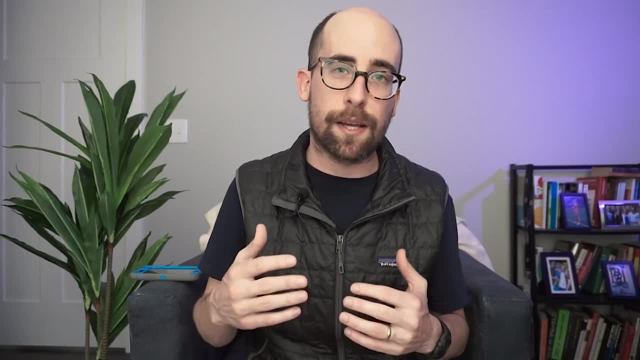 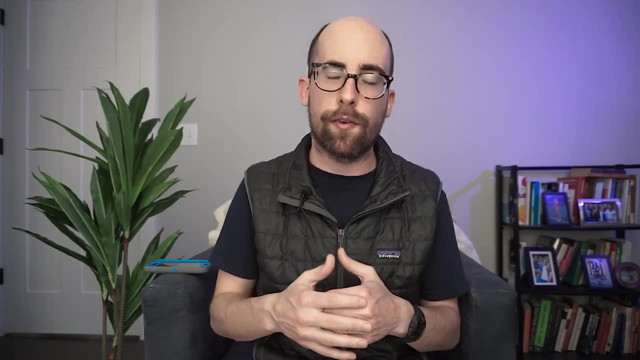 for a reason, And that is because it's really hard And I don't think it's completely passive. I think it's tempting to see monthly recurring revenue for a product that you've built once as passive. But I think the reality of owning and operating a SAS is that you have customers to speak. 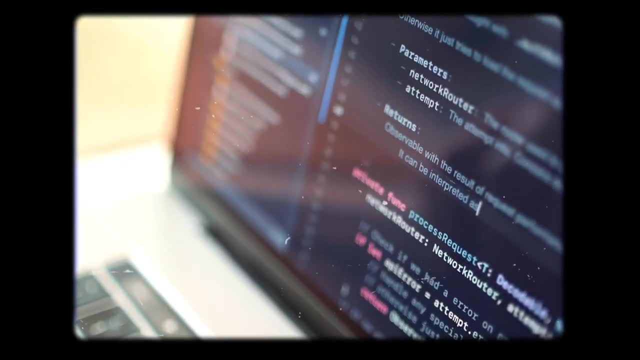 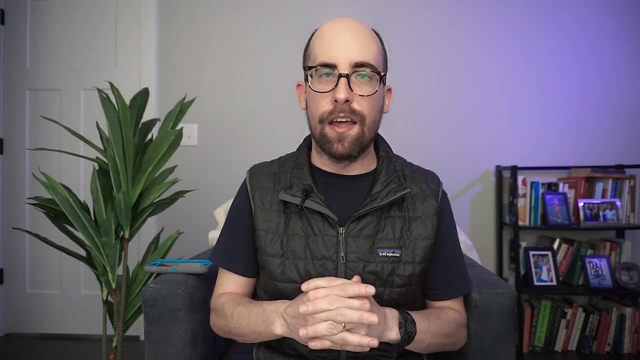 with and deal with. You have bugs to fix, Hopefully you have new features to add and you're looking for ways to compete in your market, And so I don't think running a SAS is completely passive. If it were, then Dropbox wouldn't have to hire any engineers, right? 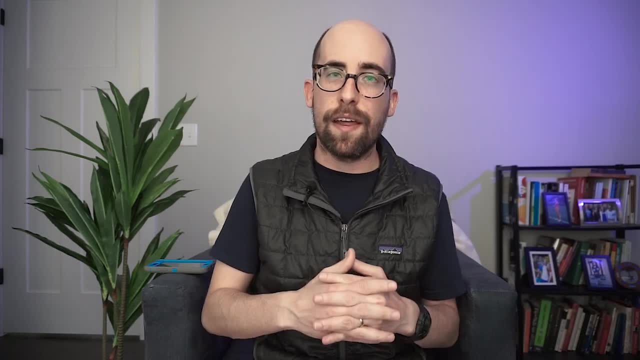 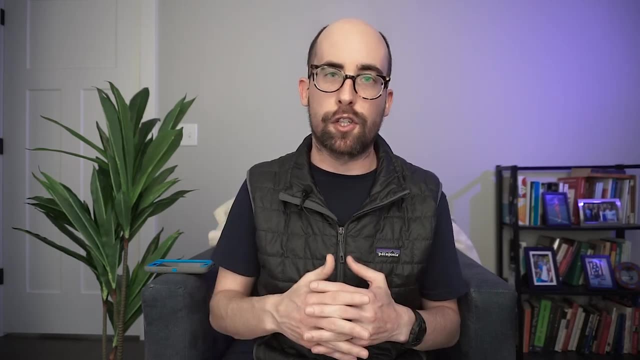 So I think it's just important to be realistic about the challenges of this. but I think if you have a kind of small niche SAS that has a limited feature set and is pretty free from bugs and has good procedures that are outlined, then the income from a SAS could. 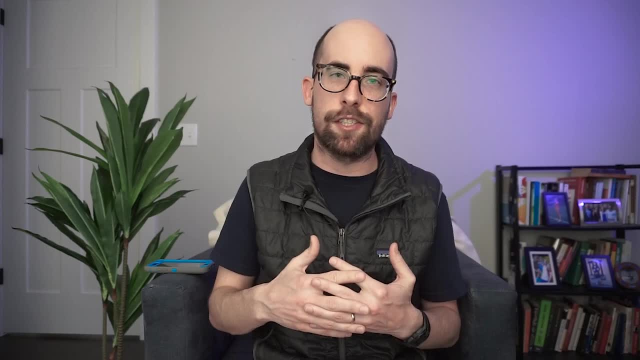 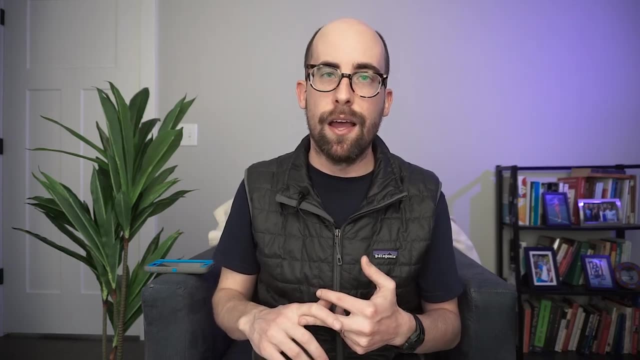 be pretty passive. So keep all these things in mind as you're considering. One other thing to consider about SAS is that it has a high time and capital risk usually, And so I would suggest really trying to validate demand as best as you can, and even charging. 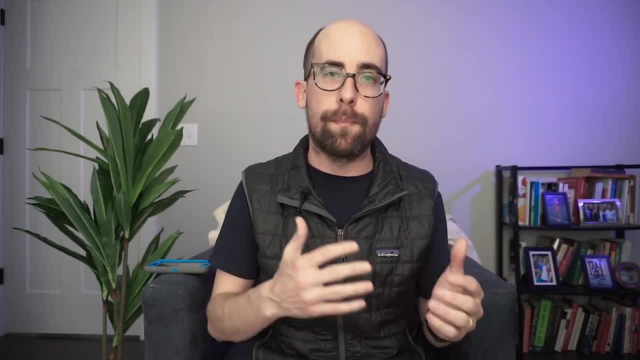 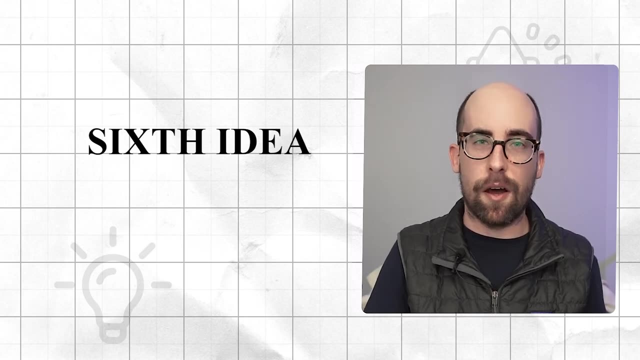 for pre-sales to ensure that people are willing to pull out their credit card to buy whatever software it is that you're selling. So just keep that in mind. Our next passive income idea is related to running a SAS, but on a smaller scale, and 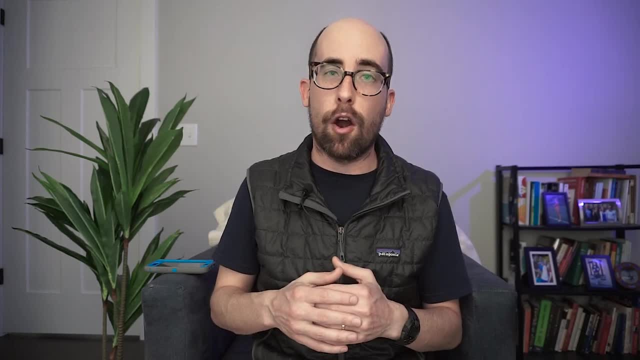 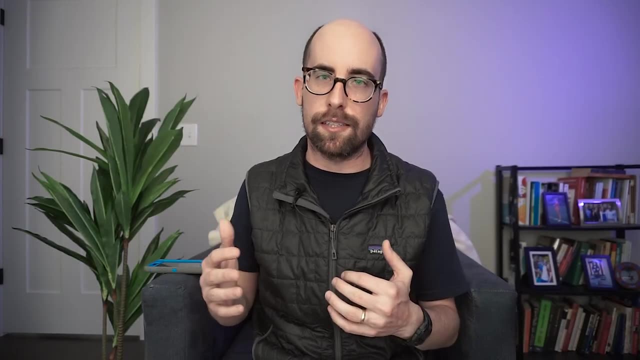 that is micro SAS, And I think this is a great option for people that are interested in selling software but maybe don't want the hassle or the headache Or the scale of a fully fledged SAS app. You could sell a micro SAS, and what is an example of a micro SAS app? 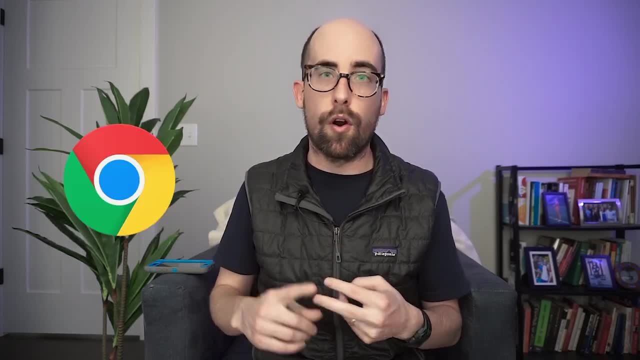 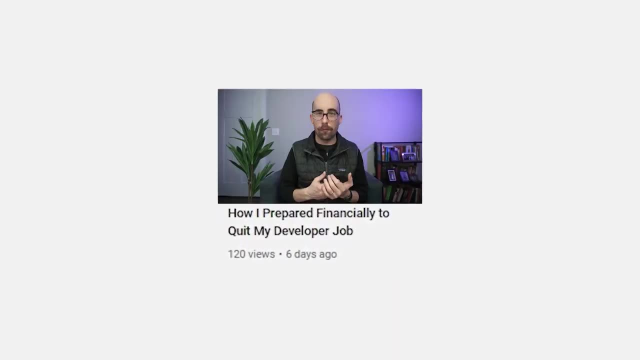 This could be a Shopify app or a GitHub app or a Chrome plugin or a Google sheets plugin. In fact, I just made a video about how my personal finance software is basically a Google sheets app. It's called tiller. It is awesome. 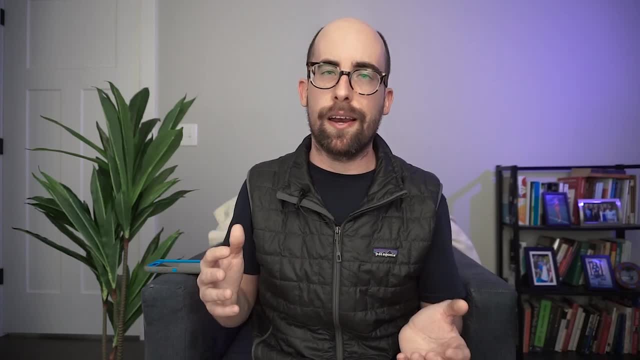 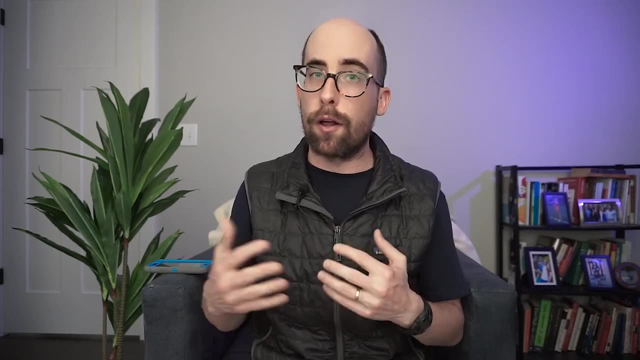 And I think there are many, many things that you could do with a Google sheets plugin, And so I would consider looking into these things. maybe look on micro, acquire or flipa and try and buy one, or try and maybe clone one or come up with a use case for yourself. 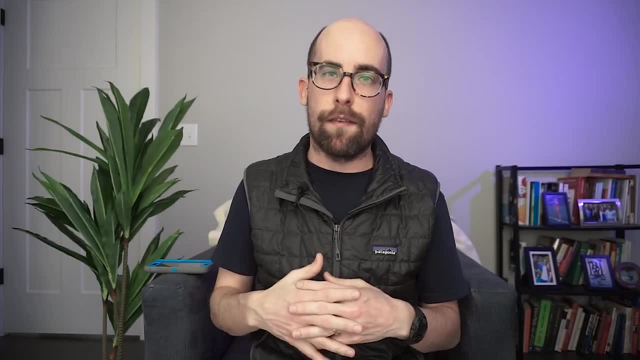 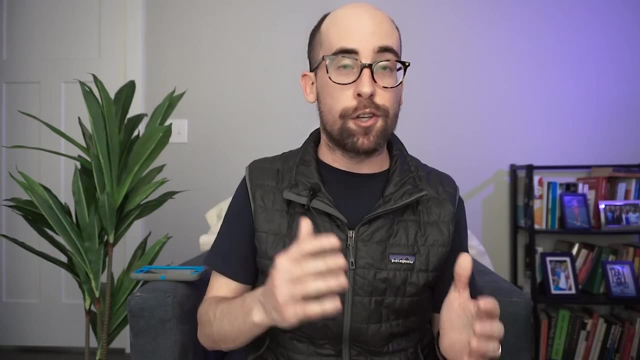 and build one. I'm personally very interested in this space, And so I might make a video in the future with updates about any particular ideas that I try to pursue. But the long story short is this shouldn't be overlooked. If you want to sell software, which I do, then I think this could be a good entry point. 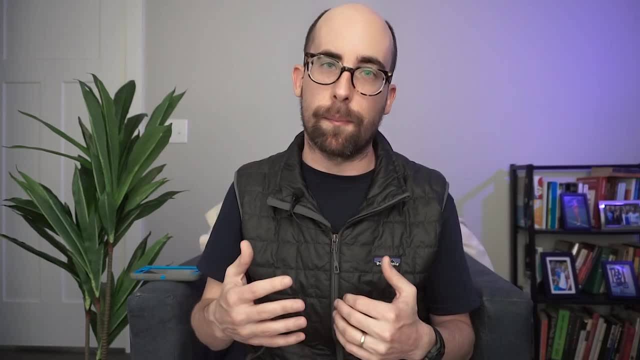 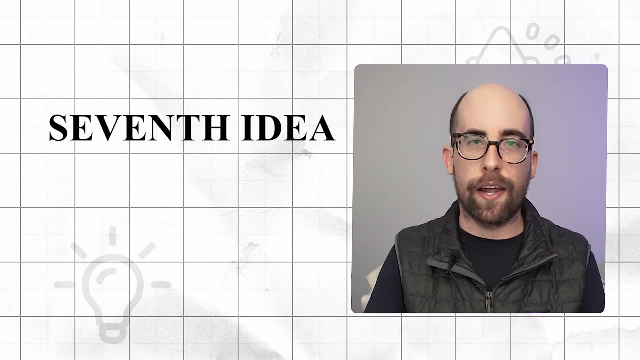 So go ahead and go out there and see what's selling and then build something. perhaps Our seventh idea. I actually saw on the contrarian thinking website. It's called credit where credit is due. Thank you to Cody Sanchez for all the great content she puts out there and this particular. 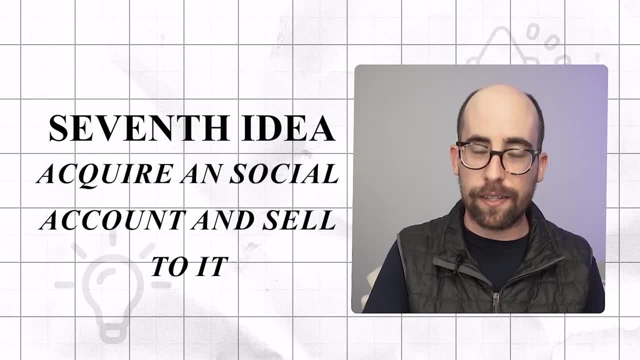 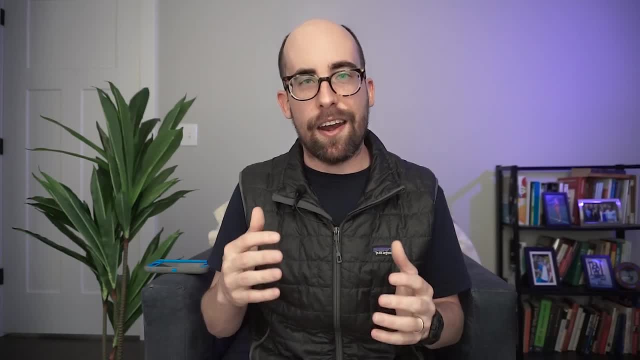 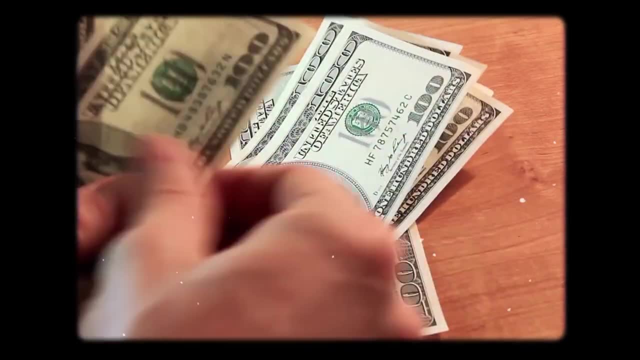 idea is acquiring a social account and then using that account to either sell things directly to the audience or to use affiliate. So I mentioned that having an audience is key, and I found that building an audience is a very long, hard game, And so you can potentially pay in order to skip some of those hard steps and just get. 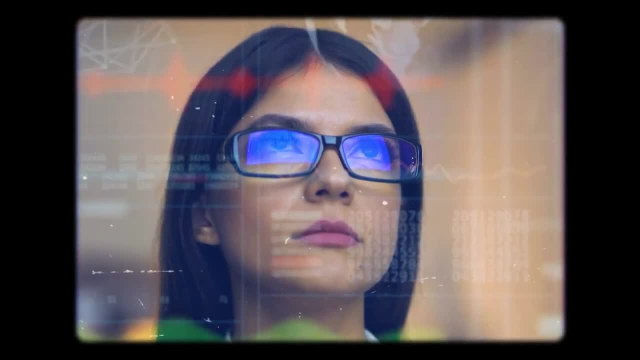 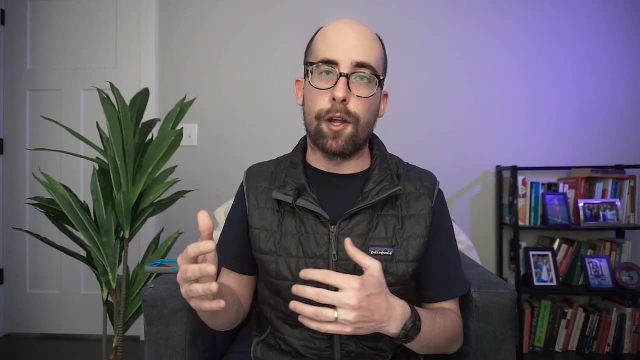 the audience. You're basically paying the person that's done all the work to build the audience, And so you can go out and maybe acquire a Facebook group or an Instagram account, And then you could- assuming you are targeting the right niche- sell products that are related. 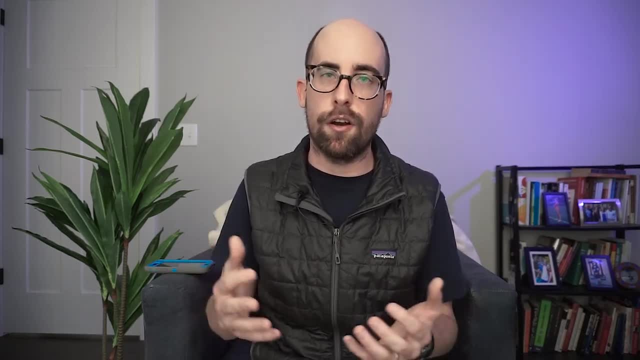 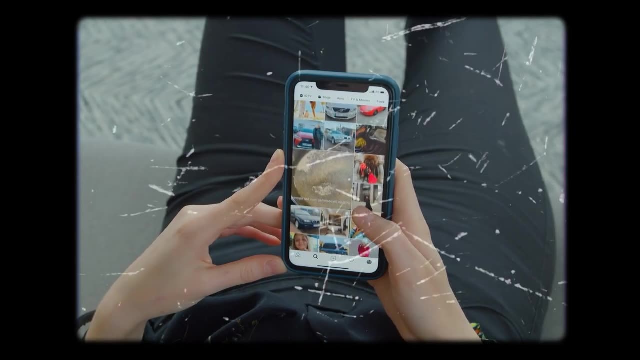 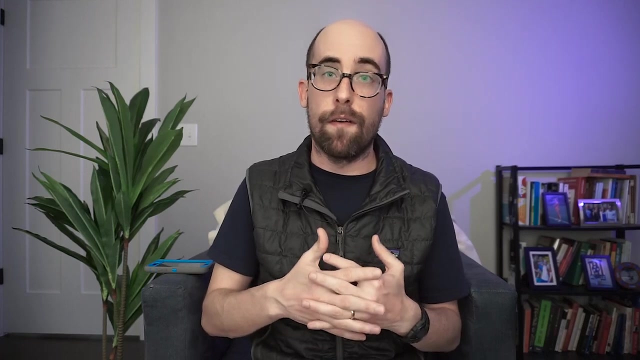 to that niche. So let's say me, for example: I'm a software engineer, I feel like I understand software engineers, And so I could go out and buy- hopefully maybe an Instagram account that is targeted toward developers, And then maybe I can come up with my own courses to sell them, or sell existing courses or have 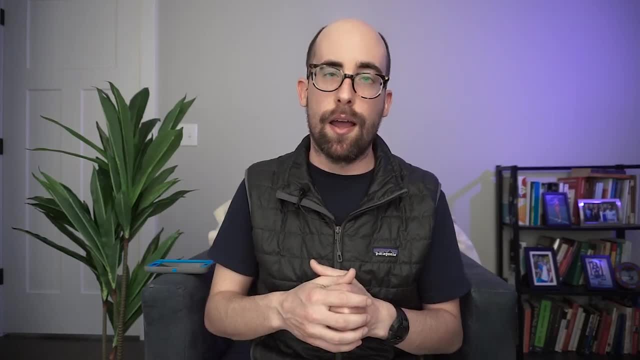 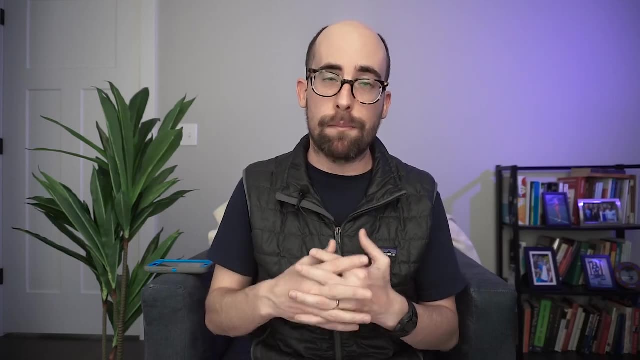 affiliate links to other courses, like West Boss, for example, And that would be, I think, a perfectly good strategy. So this is something that developers don't talk about very much. but I've mentioned a few times acquisition. I think acquisition is number one, a cool idea. 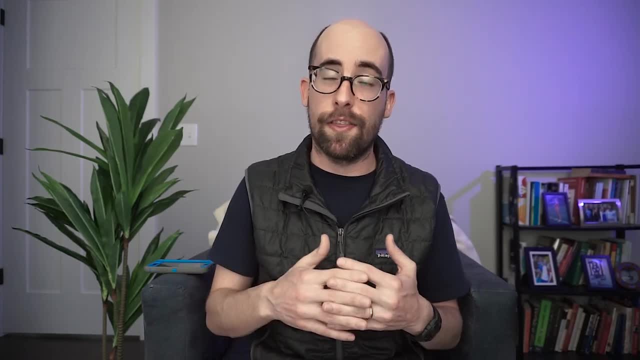 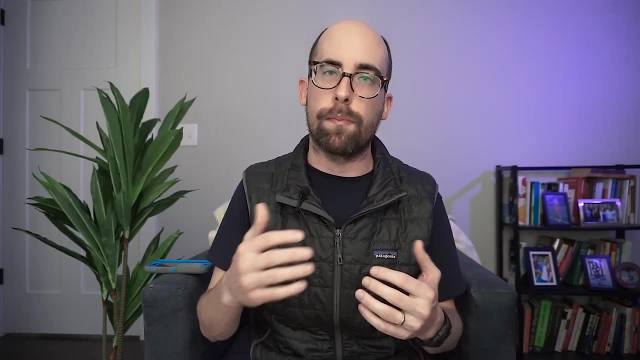 Number two can help you kind of skip that validation step and kind of hit the ground running. If you can come and bring ideas of how you might improve something to a product or service, that could be a very good option. So consider this when you're thinking about how to build passive income. 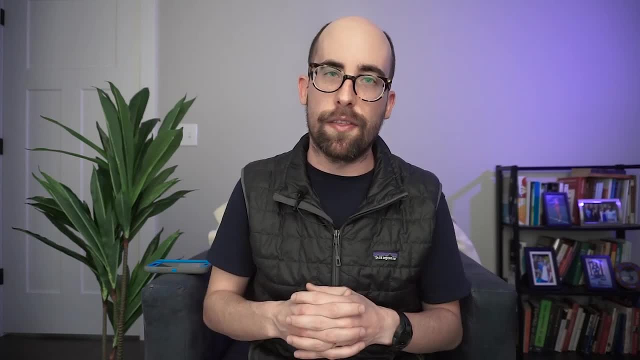 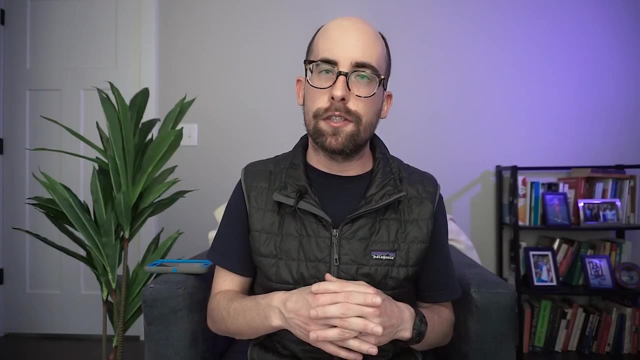 Our eighth idea is merch, And merch is pretty self-explanatory, but the thing about it is it's not completely passive, So you have to get orders and then pick items, fulfill them, ship them, And so there's some work that comes with this, but I think there are probably some. third, 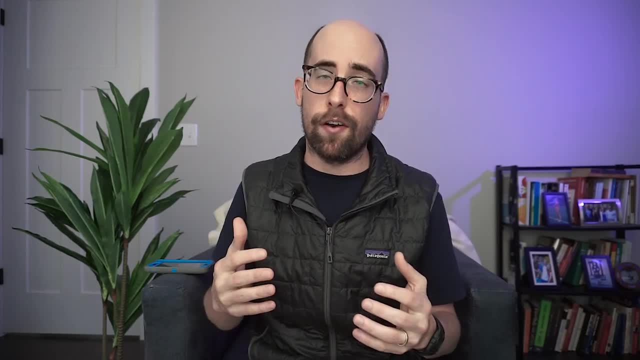 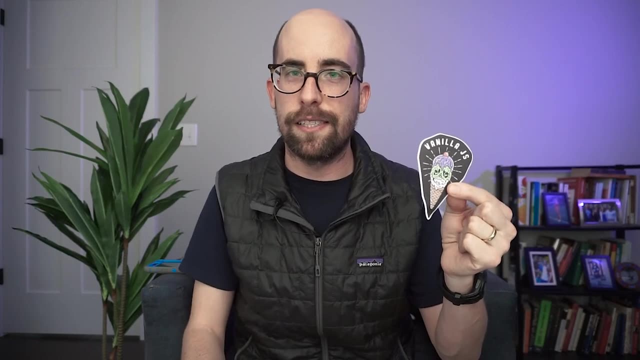 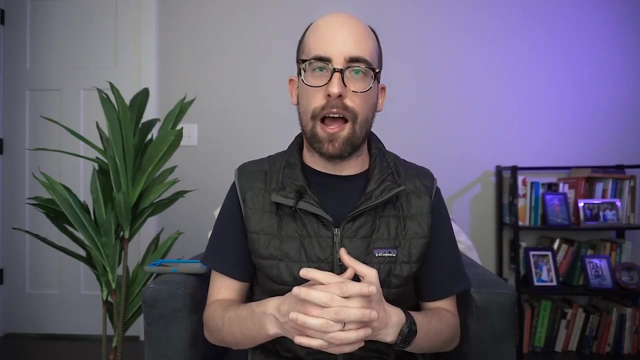 parties out there. that can make it a little bit more tenable. My favorite example of a developer who's done this is West Boss and his stickers. Let me grab one. So this is one example of a sticker from a West Boss pack. So every so often he will send stickers or he'll open up his stickers and allow you to. 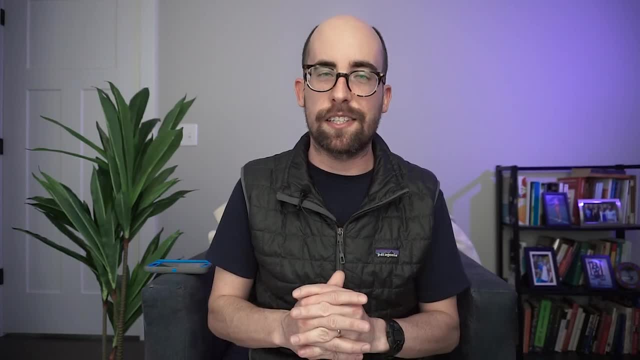 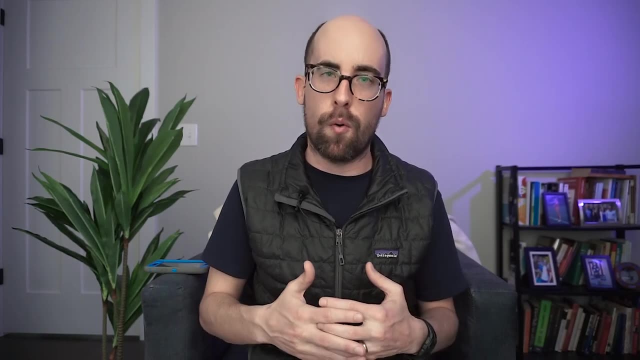 purchase them. These were $5 and they came and it's great And I think that's kind of a cool little thing you can do. that's pretty unique and fun, And so consider doing some kind of merch. I personally don't want to sell sweatshirts, but I think stuff like stickers or other items. 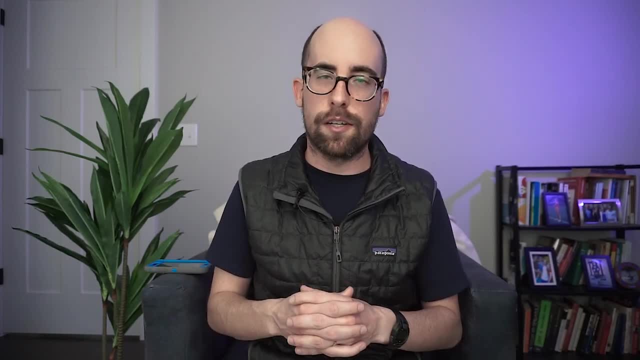 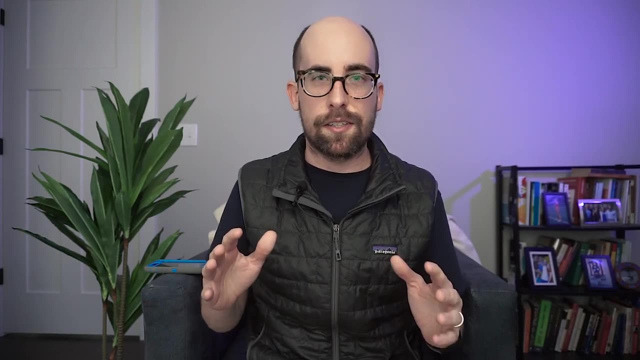 like mugs, things like that are kind of cool. So that is one more option for you. Our ninth passive income option is to offer a service on Fiverr, And I know what you're thinking. You're thinking that sounds completely not passive, but I think there is an opportunity. 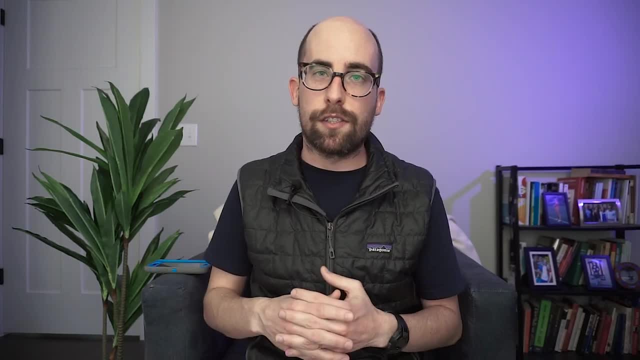 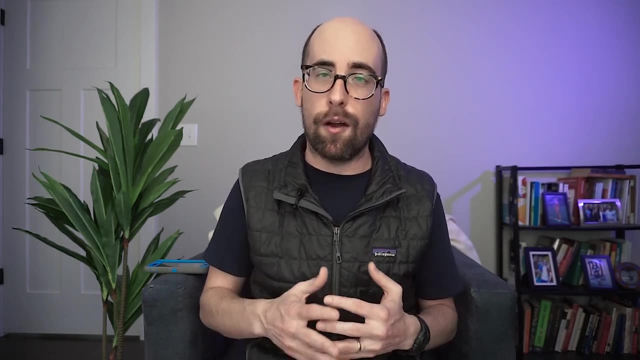 to bake some passive elements. So I think if you provide a service that you can document and kind of create a process around, then that creates an opportunity to kind of create an agency around this service. So we might call this creating a Fiverr agency. 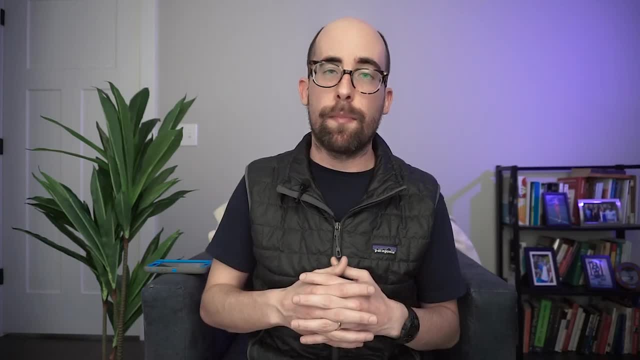 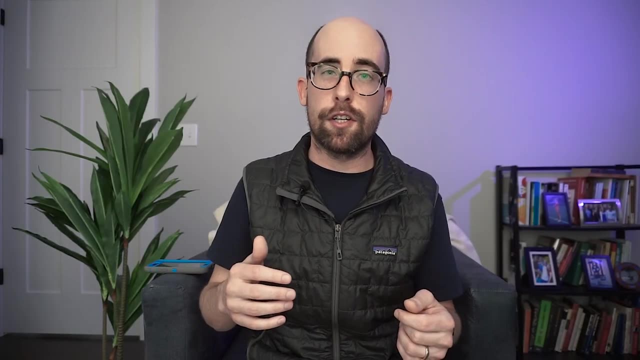 So let's say you do one page marketing sites. You can maybe develop a few of the sites on your own first and then go out and hire or outsource to a developer, And then you're kind of just doing biz dev or marketing or whatever, trying to get this. 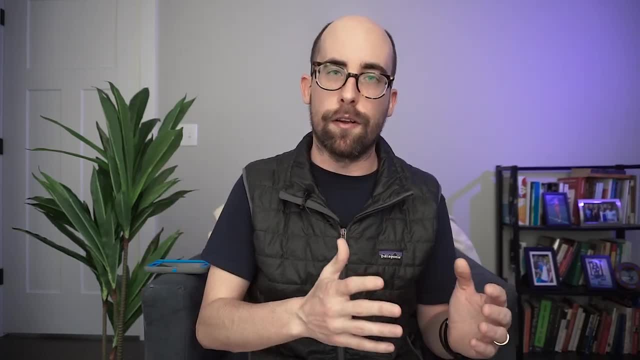 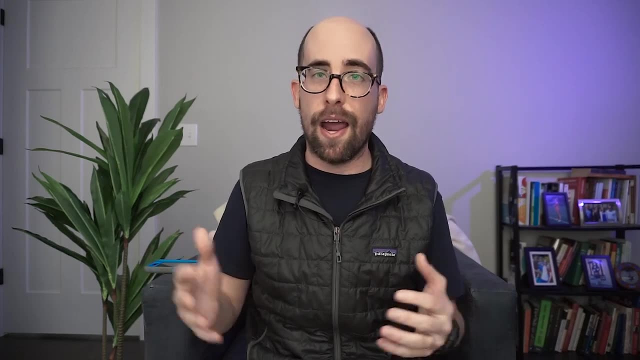 service in front of people on Fiverr, Ensuring the quality of the delivery. but then you've kind of taken yourself out of that delivery part of the process And in doing so you're able to hire and you can kind of scale this beyond yourself. 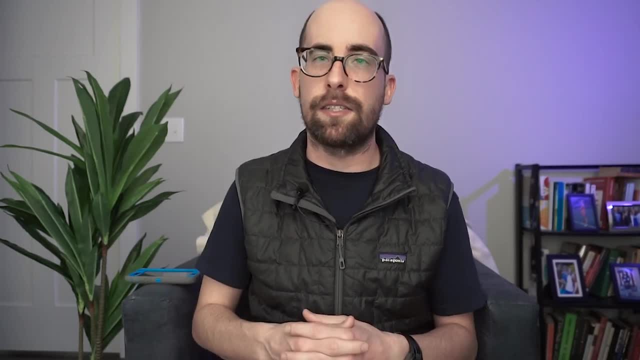 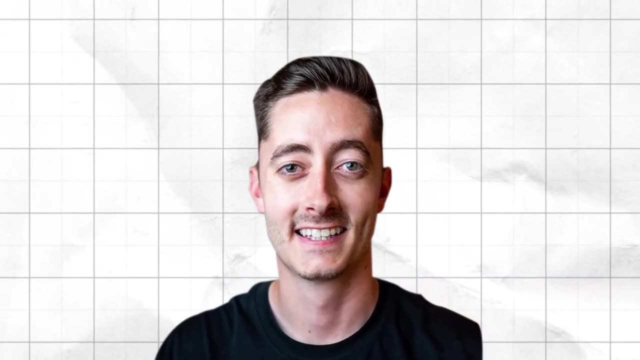 So it's not completely passive, but I think it's a cool idea and it's maybe something that I'm going to mess around with here soon. There's a great Skillshare course out there from Matt Brighton on how to have a winning Fiverr offer or service. 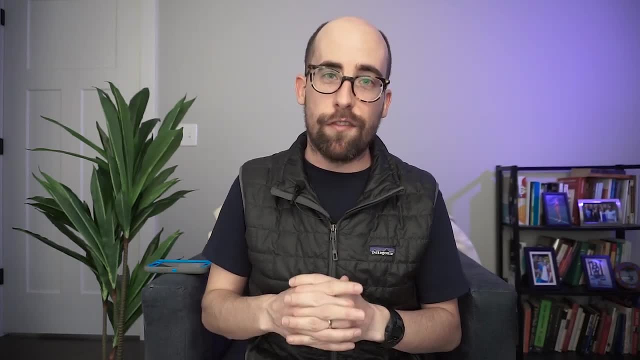 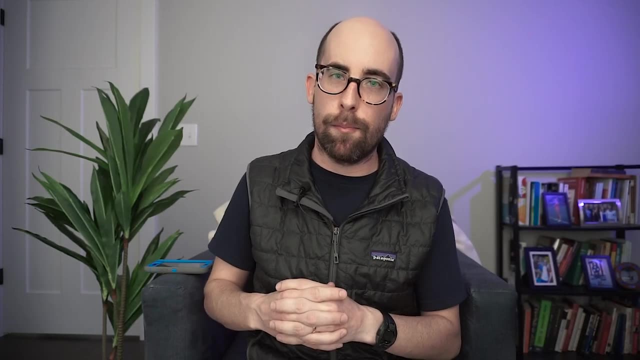 So I would suggest that, if you're at all interested. Our last two ideas are very developer-y and I think they're pretty cool. Number 10 is a component library, So I think the best known example of this is Tailwind UI, So you may be familiar with Tailwind CSS and the guys that created it. 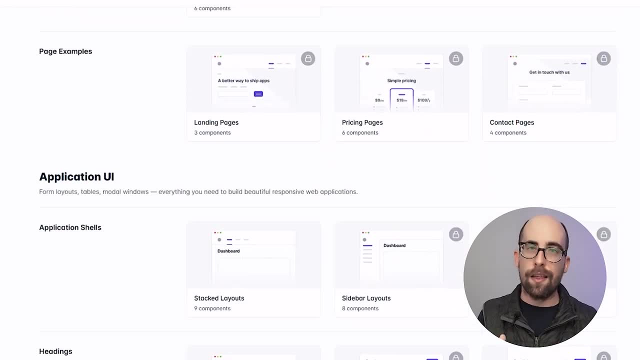 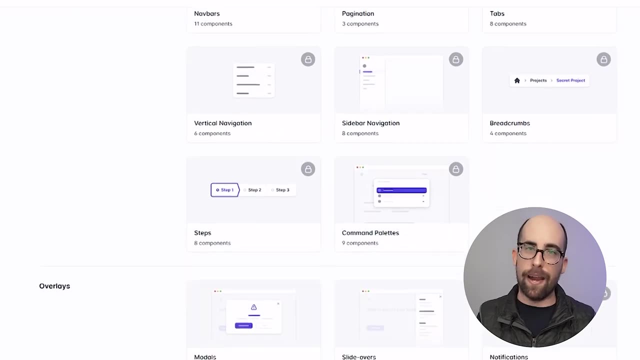 They also created these UI library components that you can buy additionally and kind of use with Tailwind. So Tailwind is free to use it's open source, but then the components are paid, And so I think that's a pretty interesting way to monetize a group of people that are 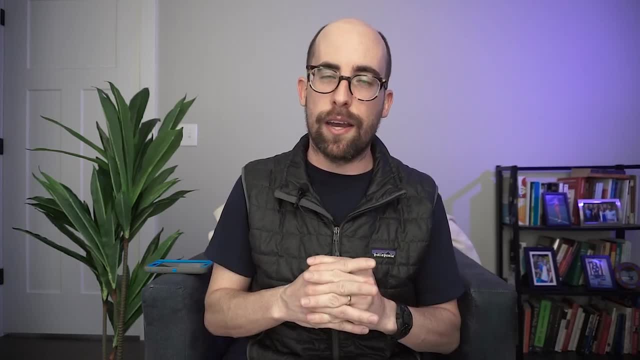 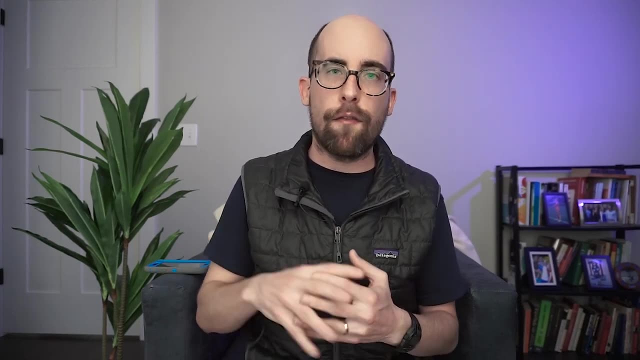 already using and really like Tailwind And the people that created it. They already have huge followings, but even if you're not them, I think there's a lot of opportunity to create components and potentially sell them. So if you have a group of related components that you've maybe used in a project, you can. 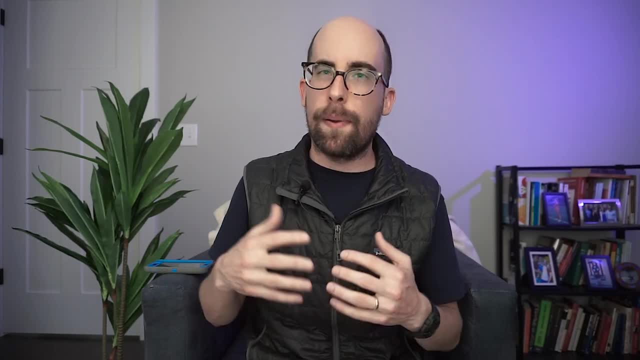 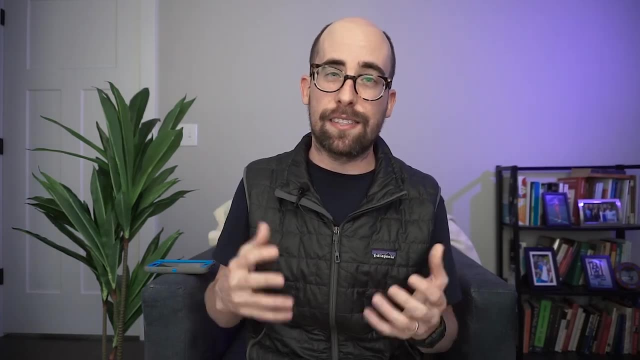 kind of pull them out and then either put them on NPM- if there's a way to gate that- or kind of just sell a zip file of those components, And I think that would be a pretty cool way to kind of sell your sawdust. 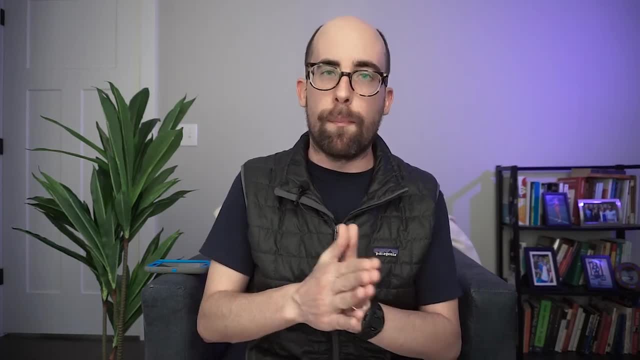 So I'm big on selling your sawdust. That just means selling things that are kind of the byproducts of things that you're already doing. So I think this is a very cool way of doing that, assuming you can kind of have either. 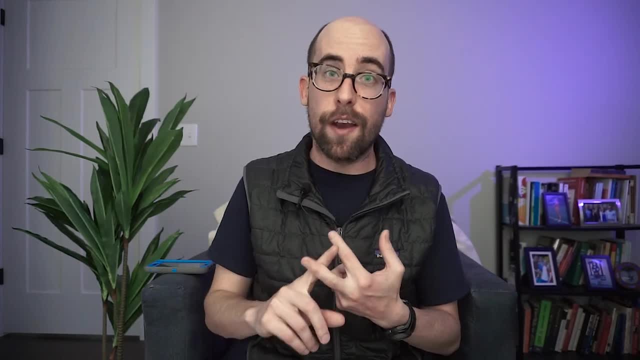 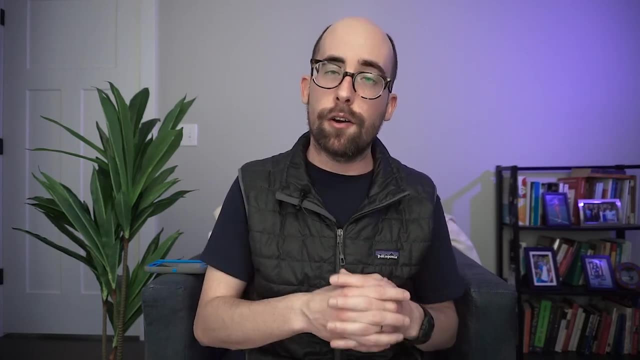 a high utility component library or high design fidelity component library? ideally both, But I would consider doing this. If you have a side project that you've done a lot of custom development for, consider how you can extract the components and maybe sell them. 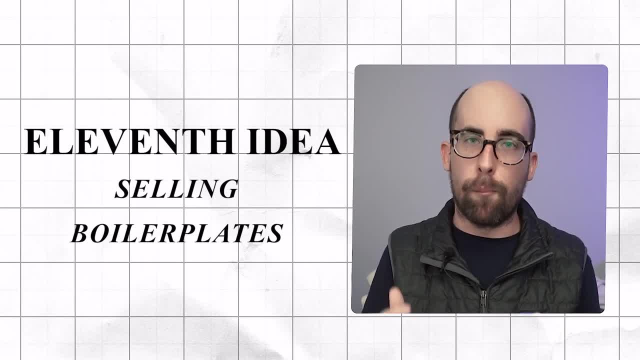 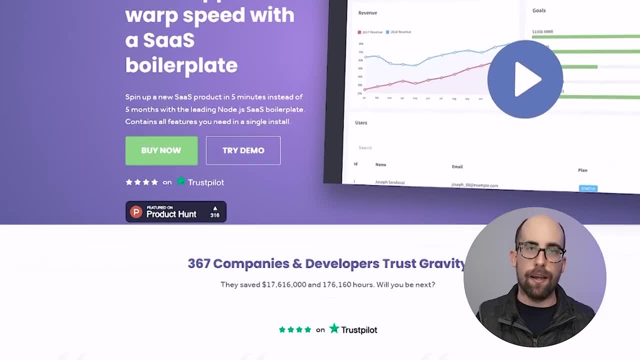 And our last idea goes right along with this, and that is selling boiler plates. So I think the best example I found of this is from this guy, Kyle Gawley, and he has this app called Gravity, And it's not really an app. 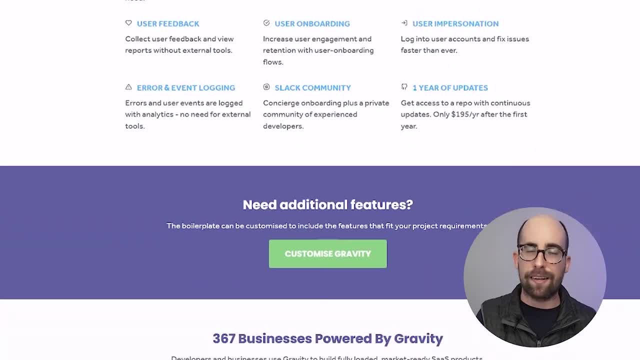 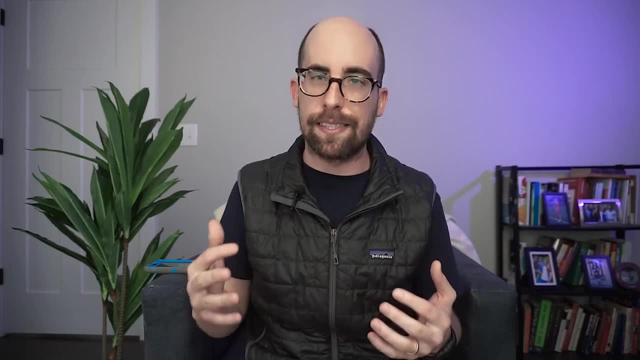 It's really just a boiler plate. It's a boiler plate for SaaS products in React and Nodejs, And so this is a great thing, because in most projects you spend a ton of time just doing the setup. I know from working in an agency myself. it's like you kick a project off and it just takes. 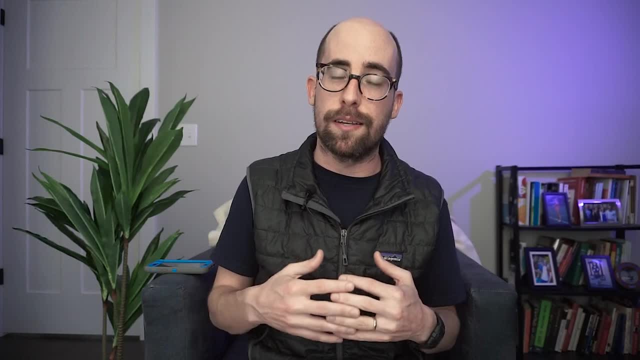 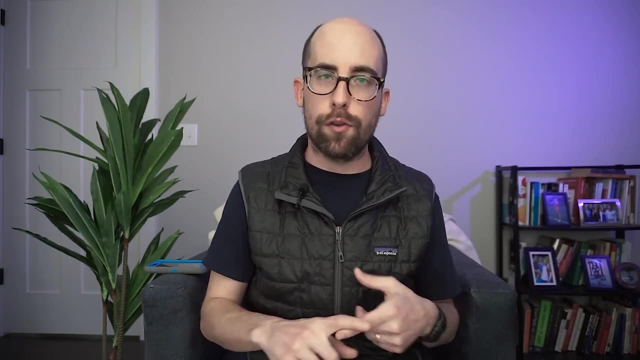 time to get all the various pieces set up And we even had boiler plates and it still takes time. So imagine how much time that a really good boiler plate is saving you from having to go and pick all the tools and pick all the technologies and do all the setup and do the.